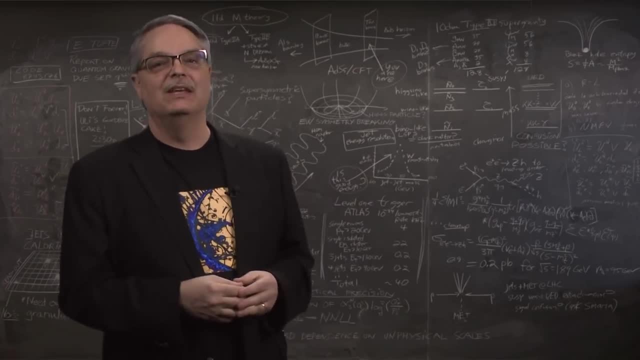 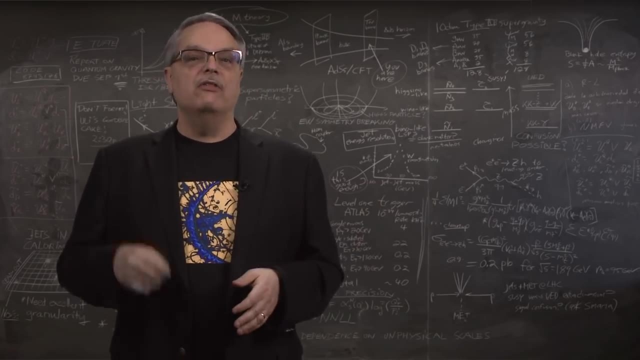 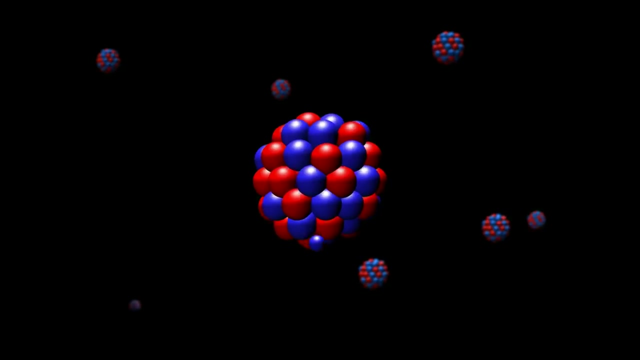 mean, come on, who would even ask such a silly question? However, there are questions that even reasonable people might ask. For instance, one question might be why the various subatomic forces have different strengths. At a distance scale of about the size of a proton, the strong nuclear force is the strongest Electromagnetism. 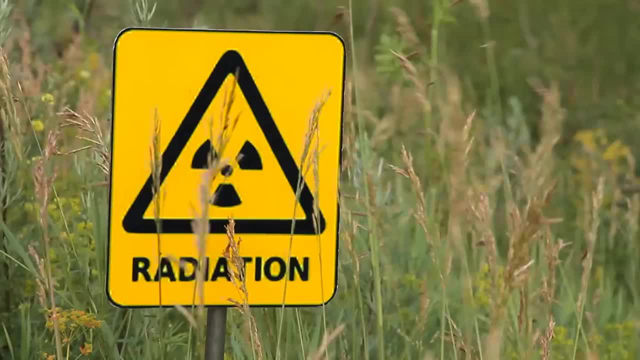 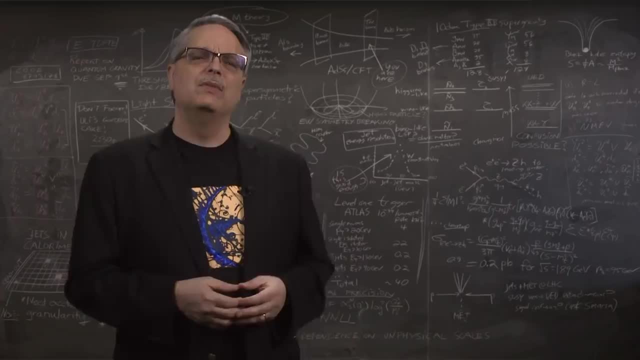 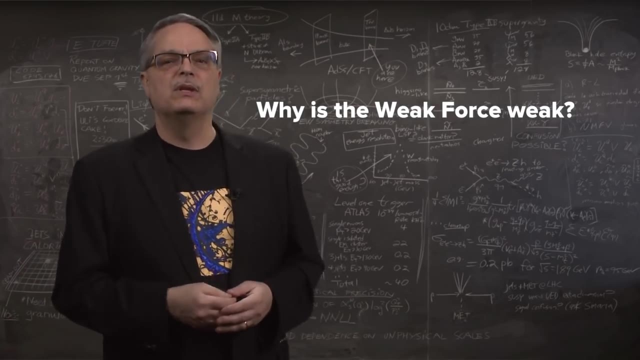 is about 1% as strong as the strong force, and the weak nuclear force is only about 0.001% as strong as the strong force. Just why these forces have the strength they do is an interesting one, and the answer differs depending on the force. So I thought I'd tell you why the weak force is so much weaker. 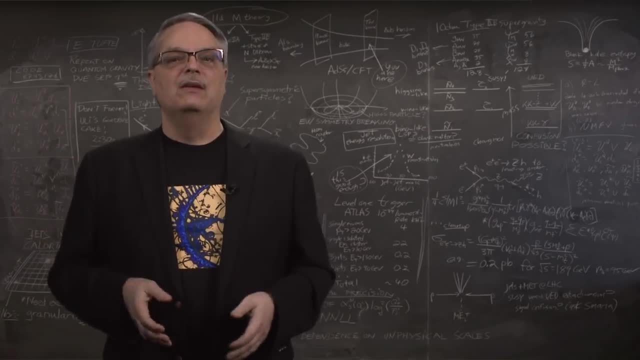 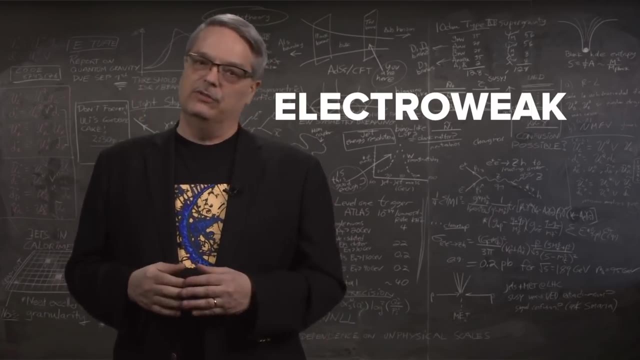 than the electromagnetic force. when they have so much in common, They've even been unified into a single force that we call the electroweak force. but that particular story I'll leave for another day. To understand what's going on, you need to remember a few things. The first thing is: 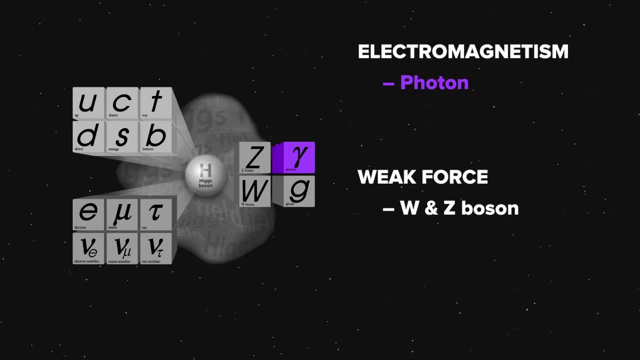 that the photon is the particle that mediates the electromagnetic force. It is massless and has no electrical charge. For the weak force, there are two particles that mediate the interaction. They are the W and Z bosons. Both of these particles are very massive. 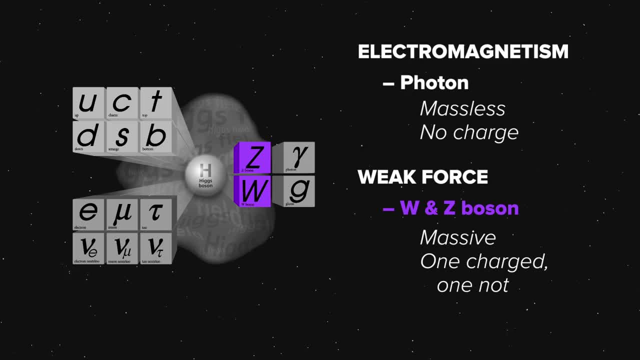 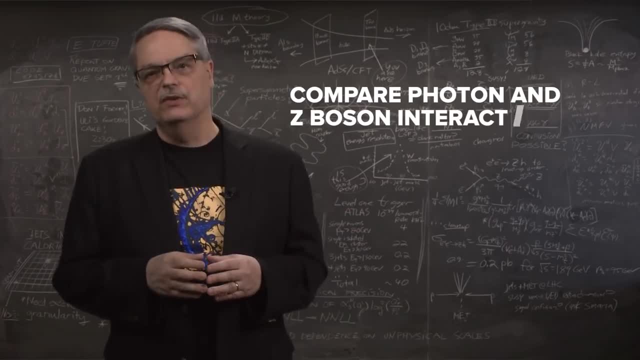 The W boson has an electric charge and the Z boson is neutral. The points I'll be making are universal, but let's just compare the photon and the Z boson for purposes of illustration, And to do that I'll describe a specific example. Let's talk about when a quark and 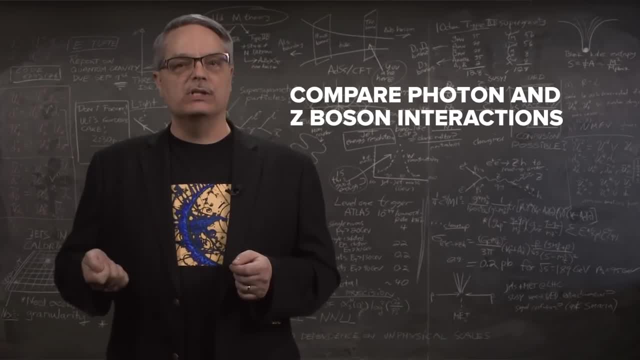 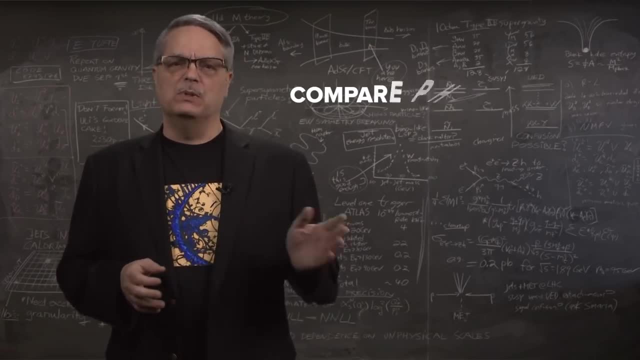 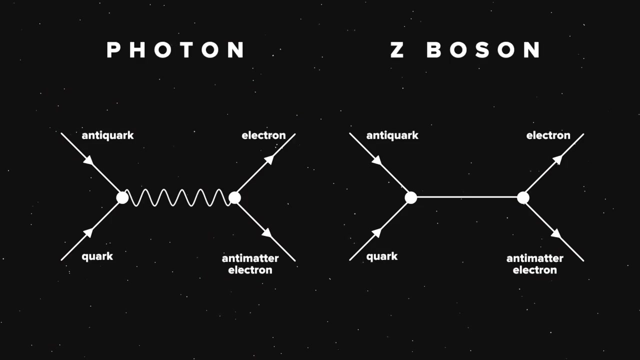 antimatter quark come together and annihilate into a force-carrying particle, which then decays into an electron and an antimatter electron. There's nothing particularly special about this particular process, it just helps me make my point. So we see here two Feynman diagrams that show what's going on On the left hand side. 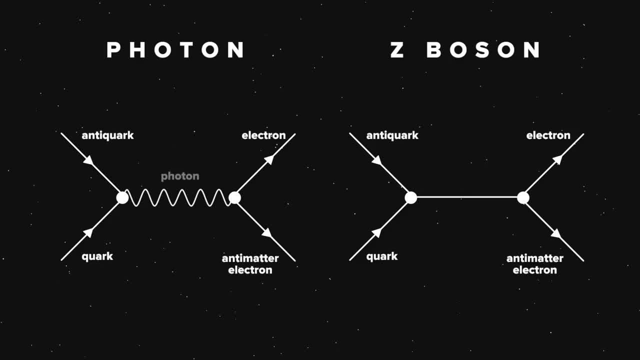 we see that quark and antiquark coming together making a photon And then decaying into the electron and antimatter electron. On the right hand side we see the same thing, but with a Z boson. They're obviously very similar. 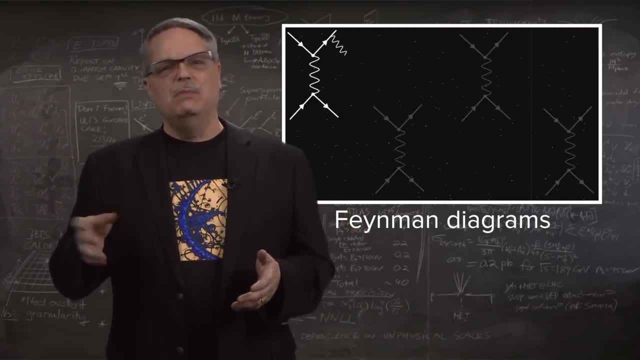 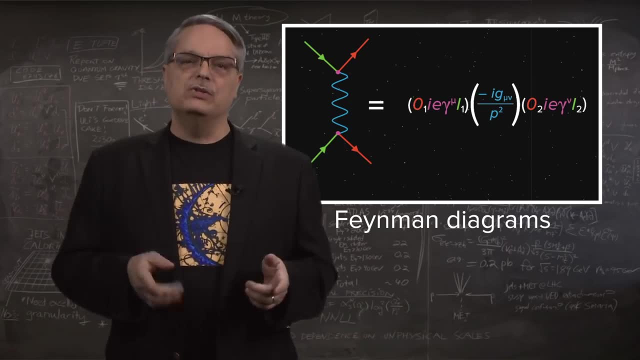 I made another video about Feynman diagrams that's relevant. It might be worth your time to watch it. While Feynman diagrams are little drawings that help visualize what's going on, they are also equations in disguise. In this case, each diagram contains seven. 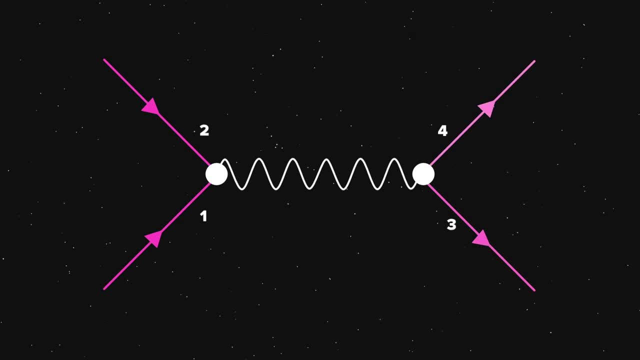 elements. There are the two incoming particles and the two outgoing particles. They're four. Then there are the two vertices where the interactions occur. That brings us to six, And finally we have the force-carrying particle. That's seven, And we see that. 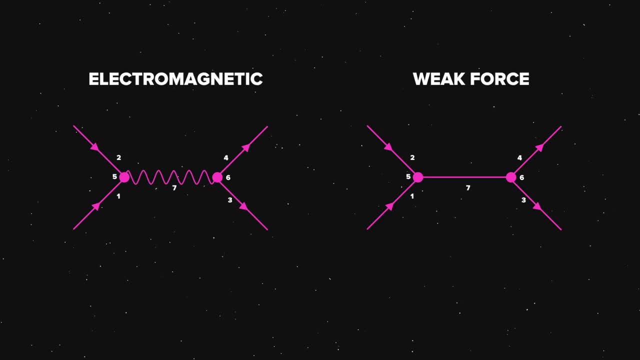 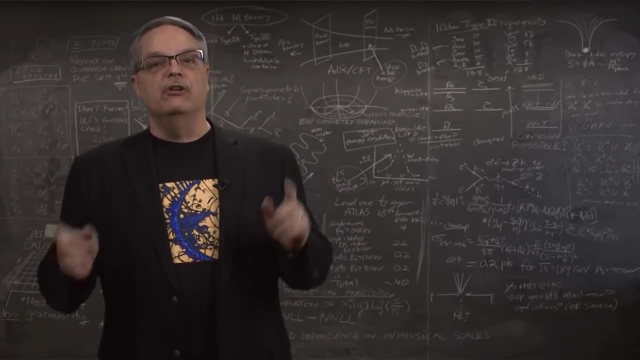 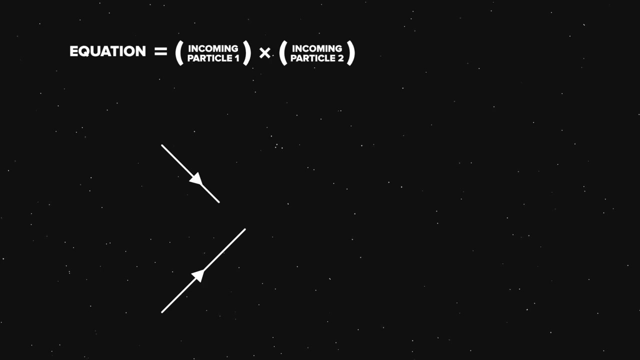 both the electromagnetic and the weak force Feynman diagrams have the same number of components. We could therefore write an equation that kind of brings that all together. For instance, we could say that the electromagnetic interaction is equal to incoming particle one times incoming particle, two times outgoing particle, two times incoming particle, three times incoming particle. 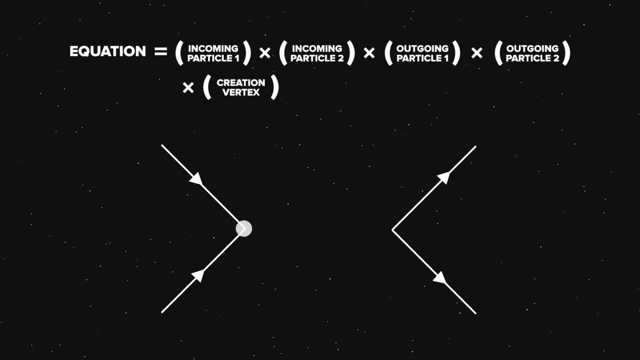 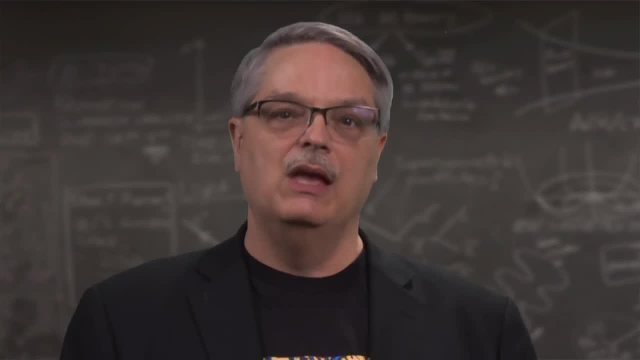 three times outgoing particle, one times outgoing particle, two times the creation vertex, times the decay vertex, times the created particle, And for the weak force we can say the same thing. So, since this equation structure governs both interactions and the diagrams are so similar, 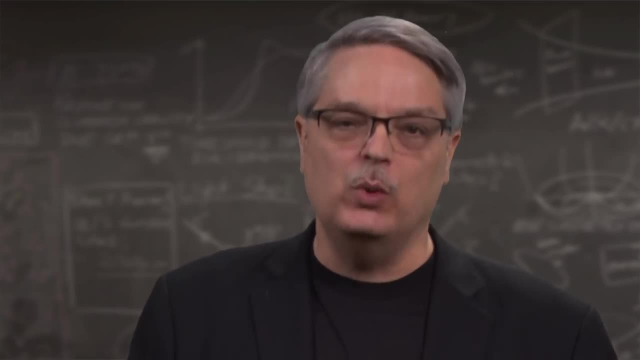 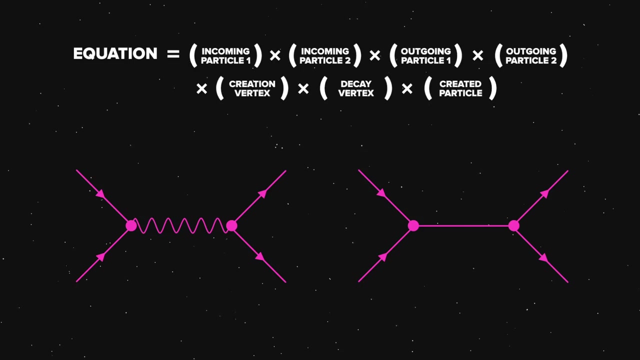 what exactly is the difference that makes the weak force so much weaker than electromagnetism? Well, we see that the incoming and outgoing particles are the same in both cases, so they can't be the source of the difference, So let's just gray them out. That means that we're left with the two vertices and 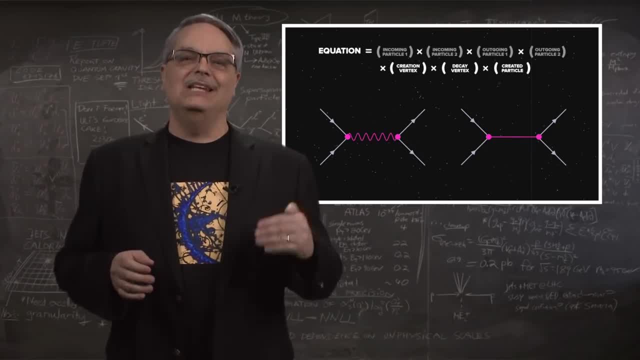 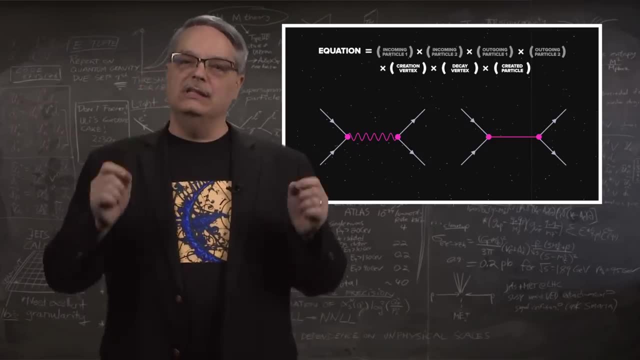 the force-carrying particle. The vertex term contains within them the charge of the interaction, and it seems pretty reasonable that the difference might occur there. After all, we know in electromagnetism that some particles have a lot of charge and others don't. However, if we actually calculate, 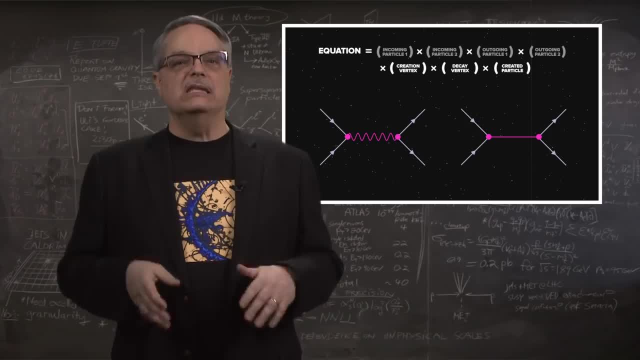 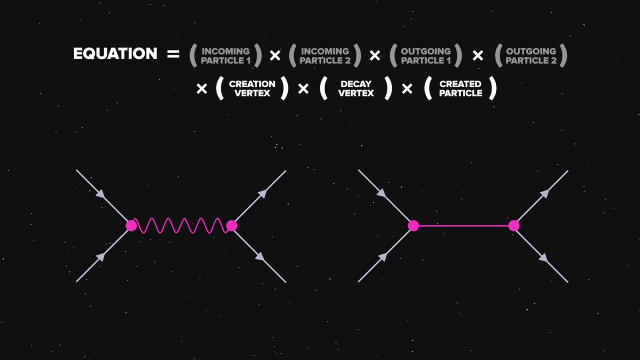 the weak force charge and the electromagnetic charge. we find that they turn out to be pretty similar in magnitude. They're not the same, so they're not the same in magnitude. So let's just gray them out. They're not the same, so don't think that. But they're not so different, So that isn't. 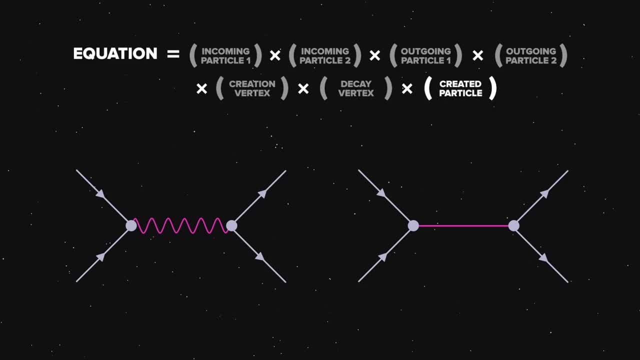 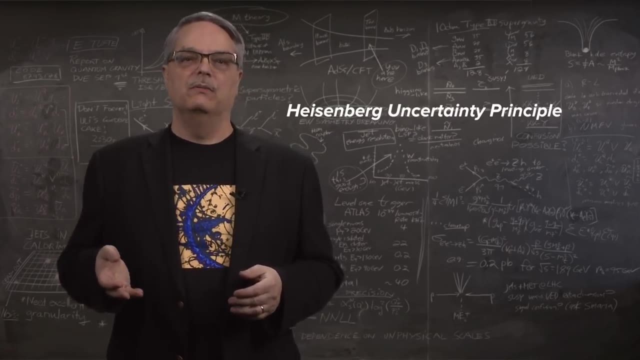 the cause either. So let's gray them out too. And that leaves us with the force-carrying term. Now the trick is to explain how the force-carrying term causes the weak force to be so weak. To take this next step, we need to talk about the Heisenberg uncertainty principle. This 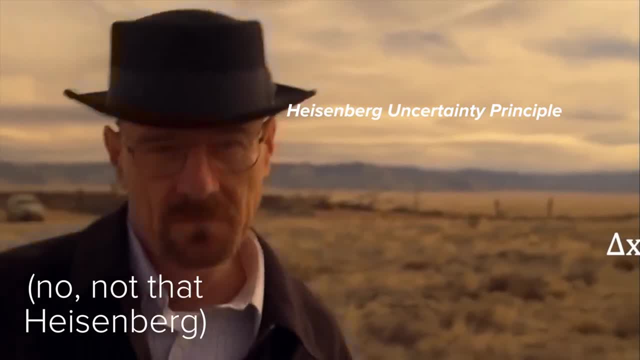 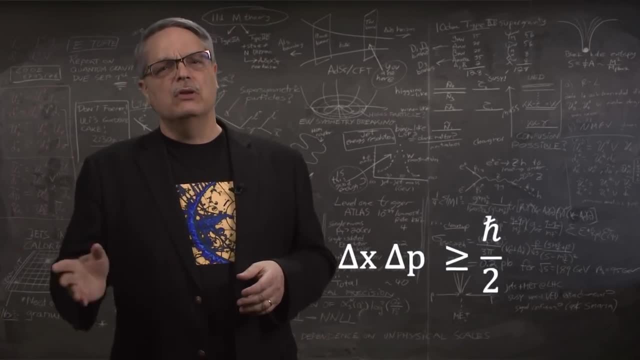 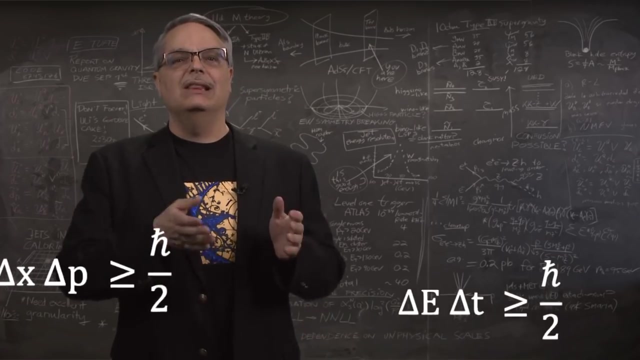 is one of the principles of quantum mechanics. It's often said that it means that you can't simultaneously measure a particle's momentum and its momentum simultaneously, And that's true. But there's another expression of the uncertainty principle that says if you look at a particle for a shorter and shorter time duration, you will have a less and less. 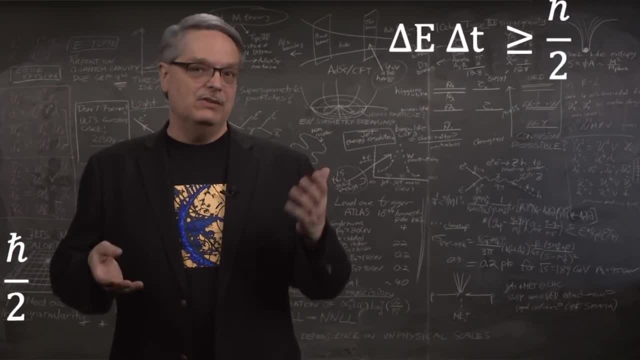 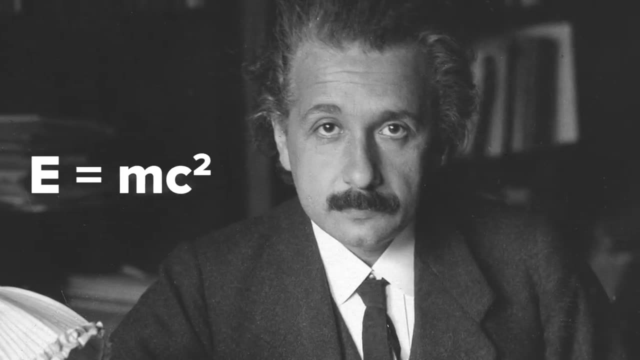 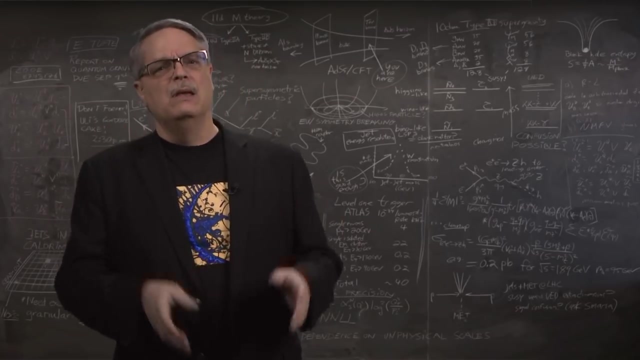 precise measurement of the particle's energy. And since energy and mass are connected via Einstein's equation, E equals mc squared. that means a particle's mass can also differ from what's expected. So that's a lot to get your head around. so let's just take a step back. Basically, what? 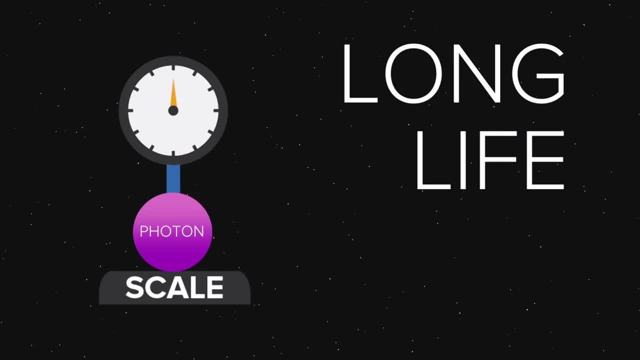 Einstein is saying is that, while a photon has zero mass, if the photon participates in an interaction that takes a very short time, for that split second, the photon might have a mass. Similarly, the Z boson has a nominal mass of 91 billion electron volts. 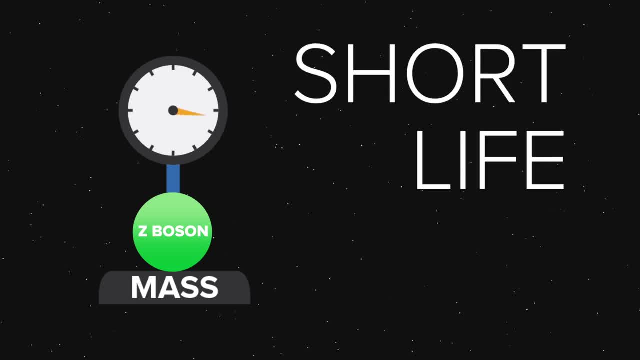 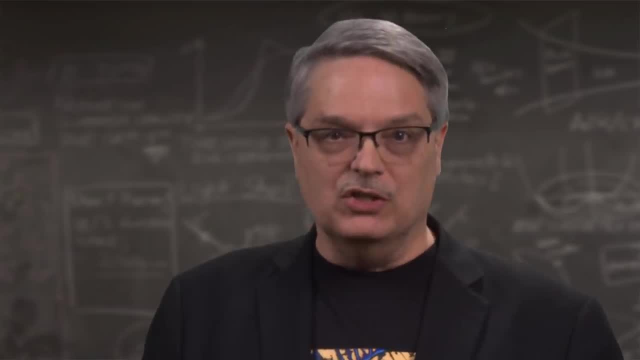 of energy, but its actual mass might differ in interactions that are very brief. This of course means that the mass of the Z boson can vary from interaction to interaction. That's a pretty mind-blowing concept, But it's also possible that the mass of the Z boson can 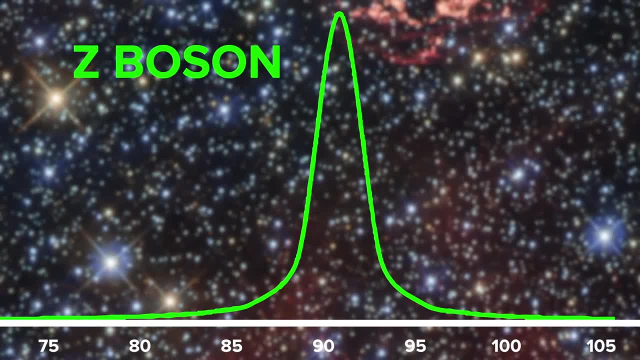 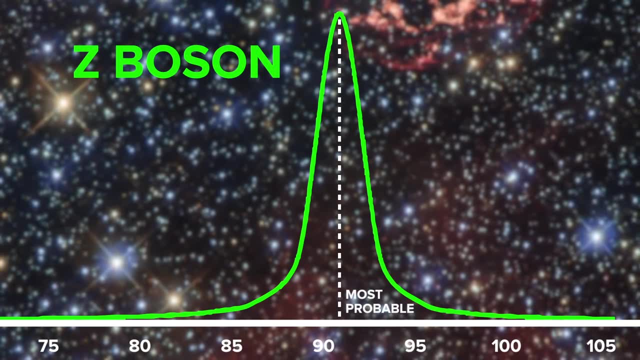 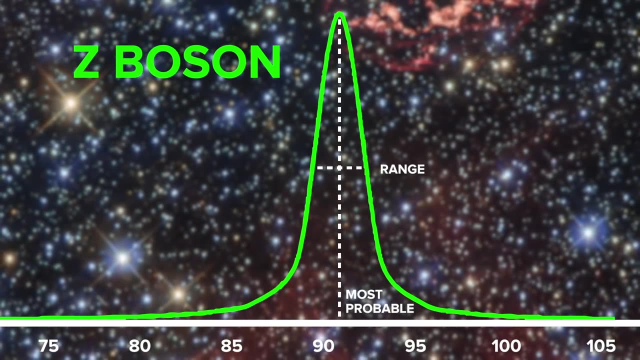 vary from interaction to interaction. In fact, we have studied the Z boson to death and while we know that its most probable mass is 91 billion electron volts, it really has a range and we can easily find it to be anywhere between 89.5 and 94.5 billion electron volts. Now, that's just the normal range, The mass. 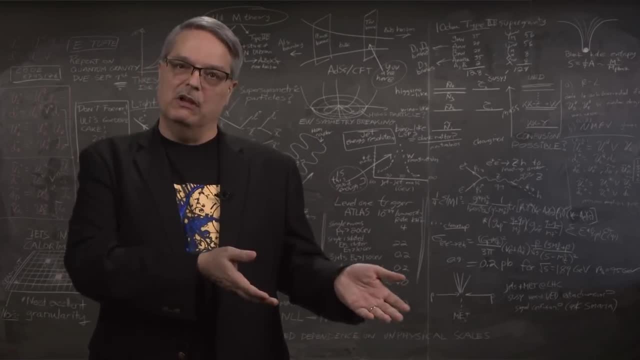 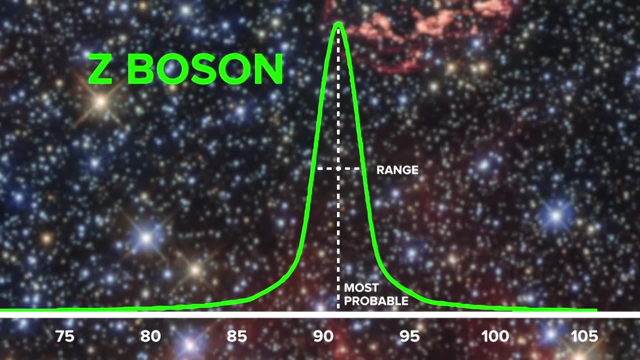 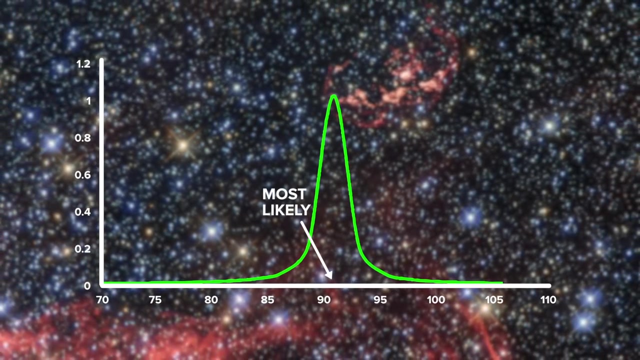 of any particular Z boson could be anywhere between zero electron volts and infinity. It's just very rare to find it outside that normal range And we can quantify how likely it is for the Z boson to have any particular mass. If the most likely mass is 91 billion electron volts, you can find it with a mass of 88.5 billion. 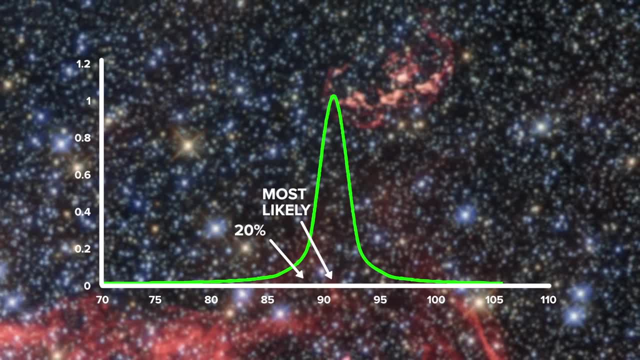 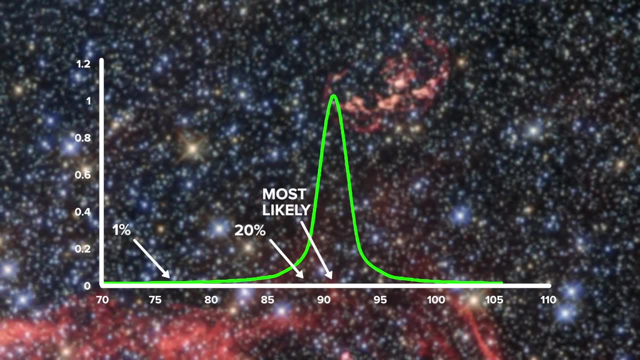 electron volts, about 20% as often. Finding it with a mass of 76 billion electron volts is only about 1% as likely, and finding it smaller than that is even more unlikely. So now we're ready to answer the question of why the weak force is so weak. Why is it? 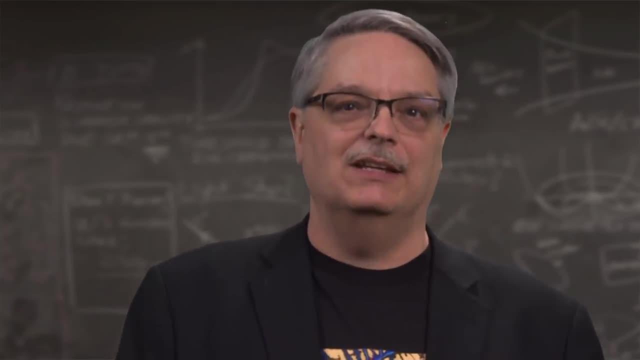 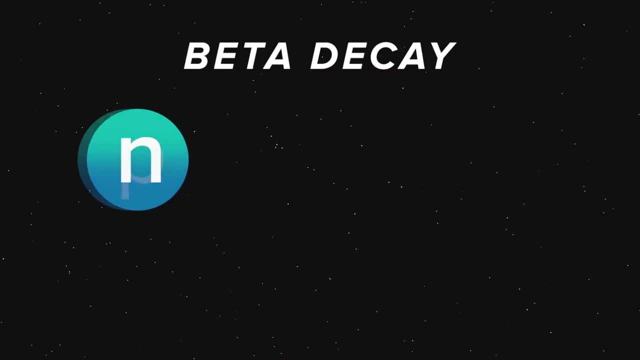 it boils down to energy. So let me hang some numbers on that. The type of radioactive decay using the weak force is called beta decay. It's when a neutron decays into a proton and emits an electron and a neutrino. An example of this: 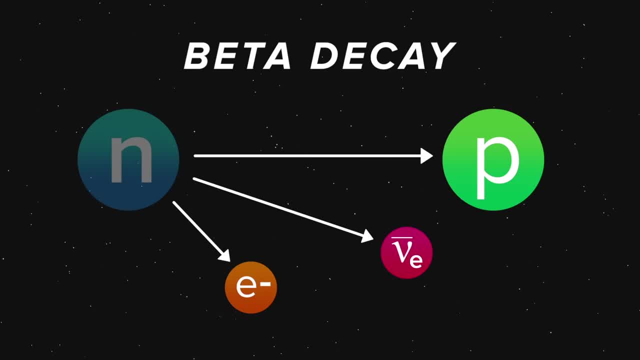 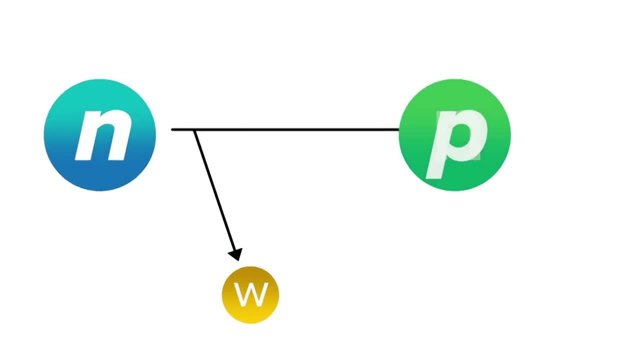 kind of decay is the carbon-14 decay that is used to date, how old some objects are. If you look at it more deeply, what you see is essentially that the neutron emits a W particle which then decays into an electron and a neutrino, And you can figure out the 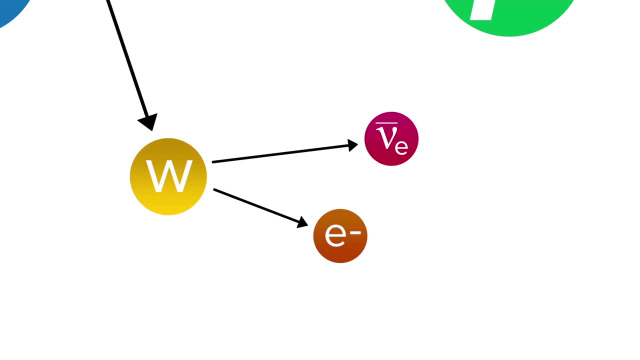 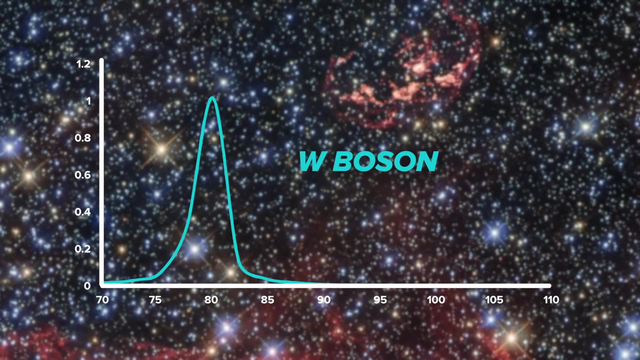 mass that this particular W particle must have. It turns out that it must have a mass of 156,000 electron volts, or in round numbers, 0.0002 billion electron volts. Now the W particle has a natural mass which is 80 billion electron volts, and its natural 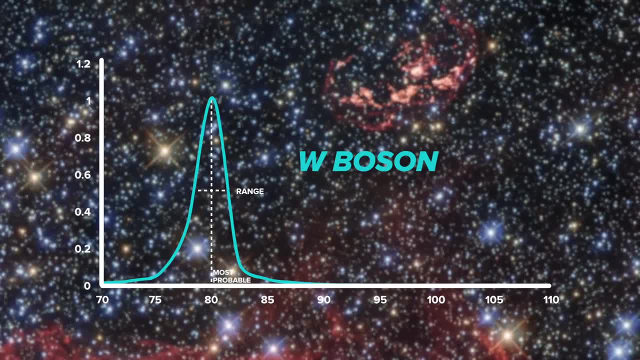 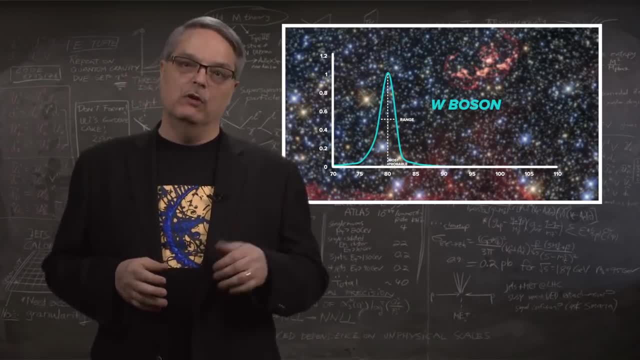 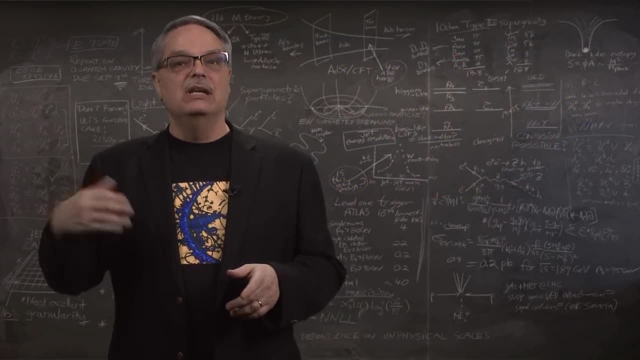 range is between 78 and 82 billion electron volts. That means that it's incredibly, stupidly, ridiculously rare for a W particle to have a mass of 0.0002 billion electron volts. It just almost never happens. And because it almost never happens, then it is exceedingly unlikely that, for example, 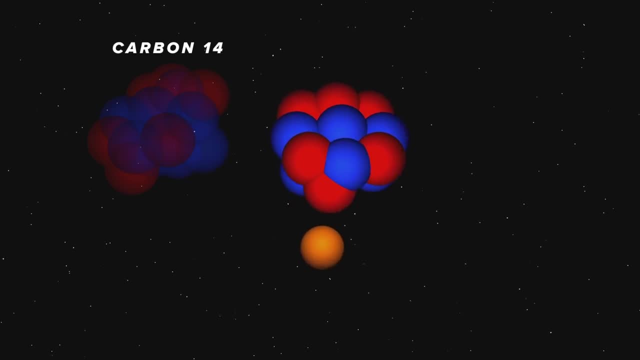 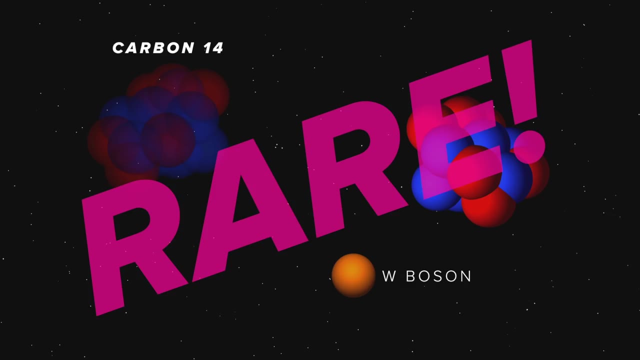 a carbon-14 nucleus will emit a W particle and decay. That means interactions that proceed by the weak force are very rare, and that is why we call the weak force weak. It's a matter of energy and the probability of making such a very light W particle. 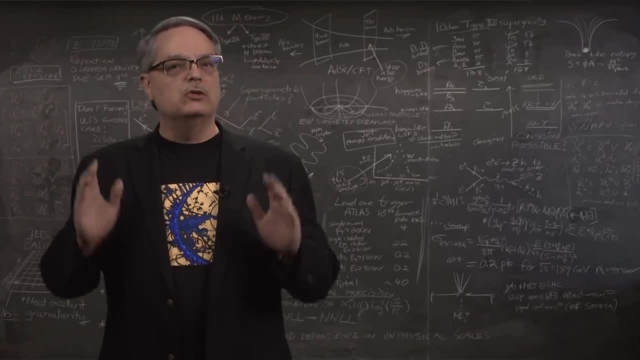 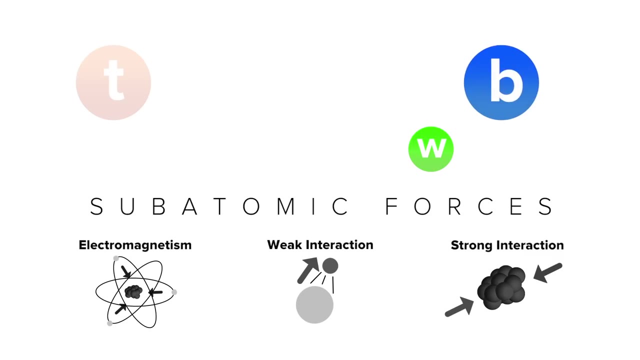 Now I wouldn't be telling you the complete story if I didn't tell you about how top quarks decay. Top quarks decay by emitting a W boson and turning into a bottom quark, And they do this decay so fast that it happens before the top quark can interact via either 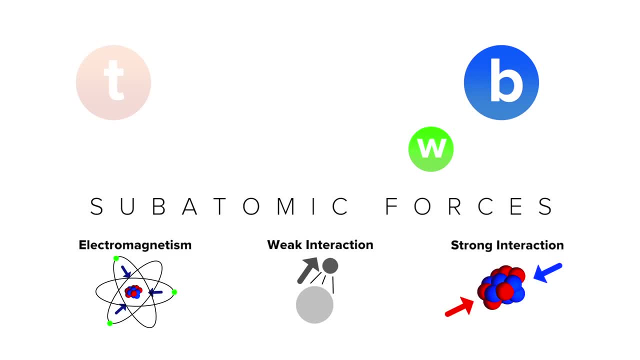 the electromagnetic force or the strong force. In fact, in top quark interactions the weak force actually happens first, which suggests that this is the strongest of the forces in that situation. Now, don't feel bad if you feel a bit confused. I've been telling you that the weak force